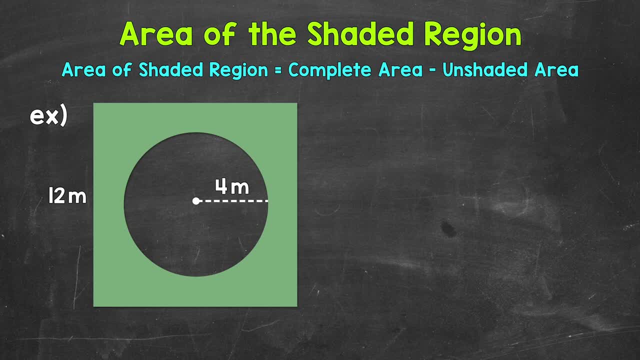 find the area of the shaded region. so the green, We do this by finding the area of the outside square and then subtracting the area of the inside circle. So I'm going to come to the side here and we're going to start with the outside square. So I will put OS for outside square and this is going. 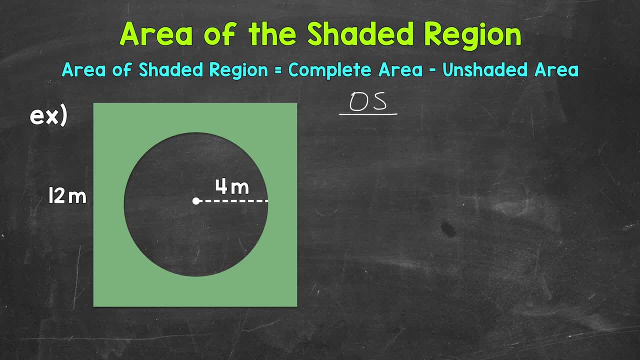 to be the complete area of that outside square. Let's use the formula: area equals a side length, squared. So for a square we can find the area by squaring a side length For the square. these sides are all 12 meters, So let's plug in 12 meters. So area equals 12 squared. 12 squared means 12 times 12.. So 12. 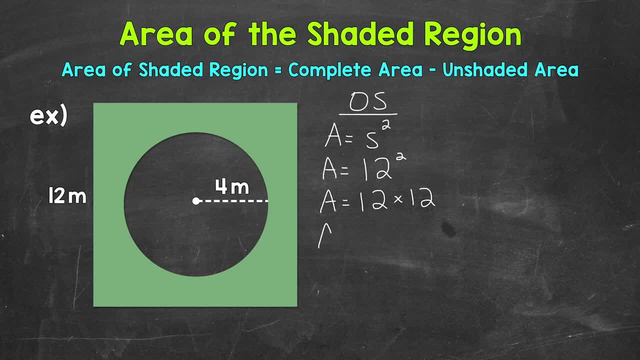 times 12.. That gives us an area of 1.5 meters. So let's plug in 12 meters. So area equals 12 squared. That gives us an area of 144 square meters. That's the complete area of the outside square. Now we 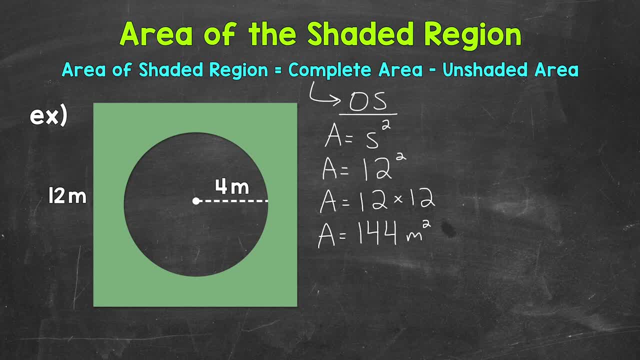 need to subtract the area of the inside circle. We need to take out the circle hole, so to speak. Let's put IC for inside circle and this is the unshaded area. Now for the area of a circle, we use the formula: area equals pi R squared, So pi times the radius squared The radius of the circle. 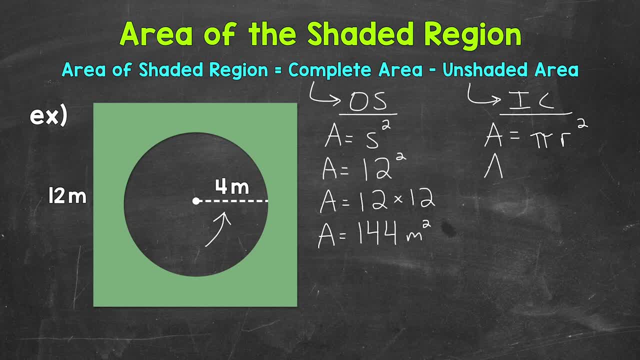 is 4 meters, So let's plug in 4 meters for the radius. so we have pi times 4 squared. 4 squared gives us 16.. 4 squared means 148.. So we can, we can change the radius, So we can change the total. square we can change the total radiusbut 4 times 4 squared we get 72 square meters. 4 squared gives us 16.. 4 squared means 42 square meters. So 4 square equals 3 squared, 4 squared of this. is 4, telling us that we're going to put A very tiny square area here. That means 21ened. So in this case, have 4 squared and that means 22.. So again, that means the whole square. If we are interested, the area equals 2. or if you want to multiply over a size, we have a triangle in. 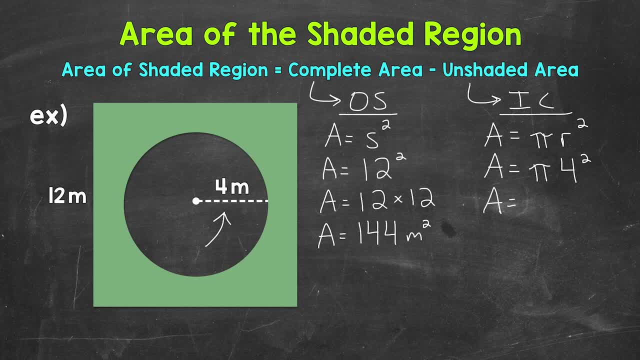 times 4.. So area equals pi times 16.. I'm going to use 3.14 for pi, which is an approximate value for pi, So we need to do 3.14 times 16 now. That gives us an approximate area of that circle. 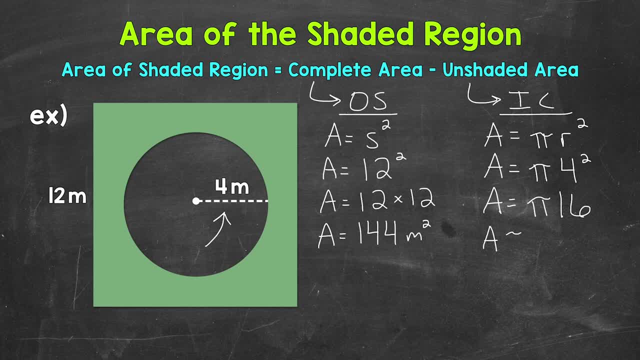 So the area is approximately 3.14 times 16.. That gives us an approximate area of 50 and 24 hundredths square meters. Now that we have the area of the outside square and the inside circle, we can find the area of the shape. 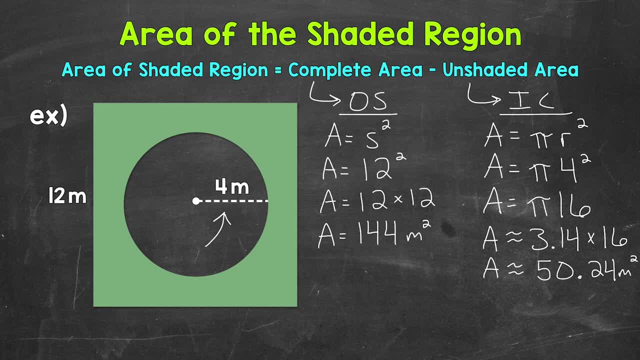 We need to take the area of the square and subtract the area of the circle, So the area of the shaded region is approximately. Remember again, the area of the circle is an approximation. It is a very close decimal value. So that is going to give us an approximate area of 50 and 24 hundredths square. 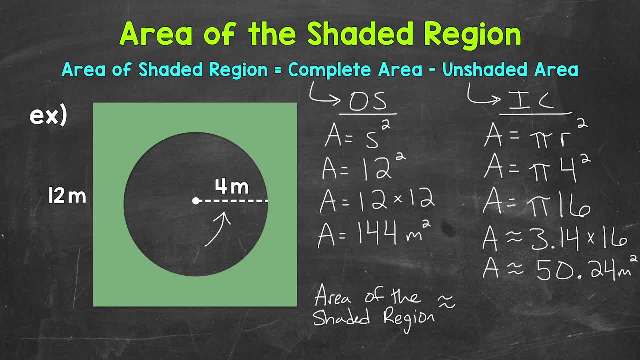 meters. So that is going to give us an approximate area of the shaded region. We have 144 square meters, the area of the square, minus 50, and 24 hundredths square meters- the area of the circle. That gives us an approximate area of 93 and 7.4 square meters. So that is going to give us an approximate area of 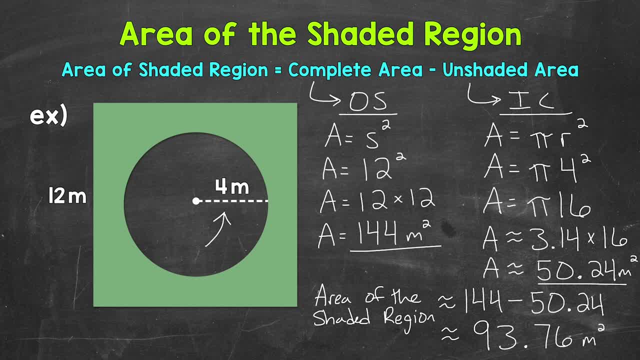 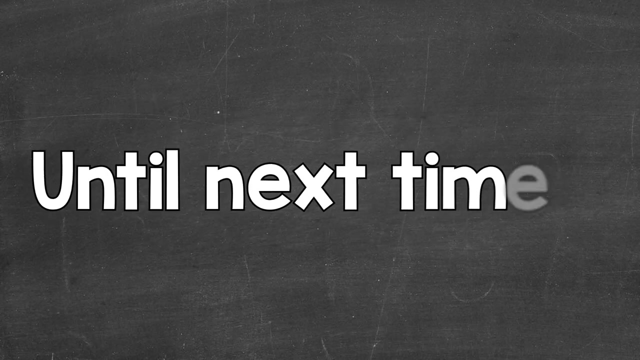 76 hundredths square meters, And this is our final answer. So there you have it. There is how to find the area of the shaded region And specifically, we had a circle inside of a square. I hope that helped. Thanks so much for watching. Until next time, peace. Subtitles by the Amaraorg community.